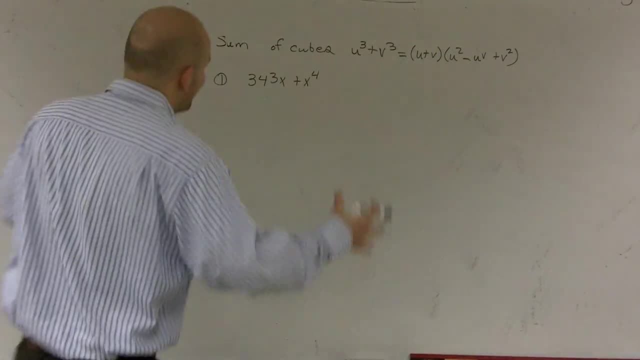 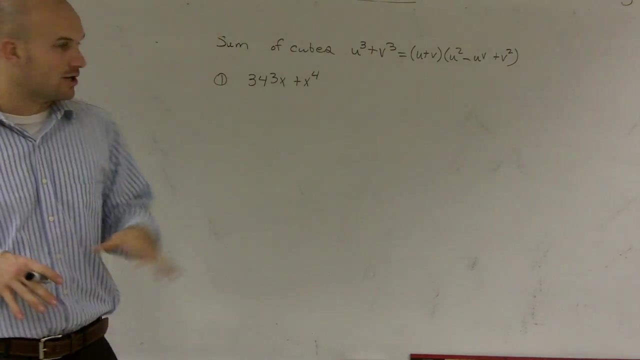 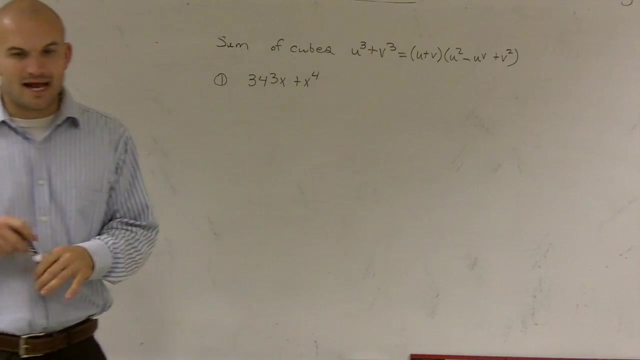 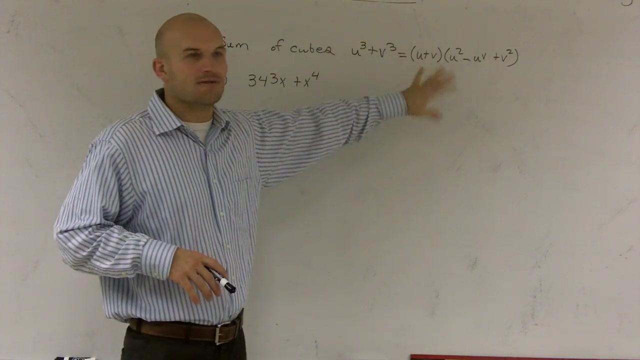 Alright, what I'd like to do is show you how to find a sum of cubes. Usually it would be the sum or difference. I'm just going to focus on the sum of cubes. So we have a problem of 343x plus x to the fourth power And it asks us to use the sum of cubes to factor. So what we want to do is- I have this little abstract kind of formula here that u cubed plus v cubed plus u plus v times u squared. 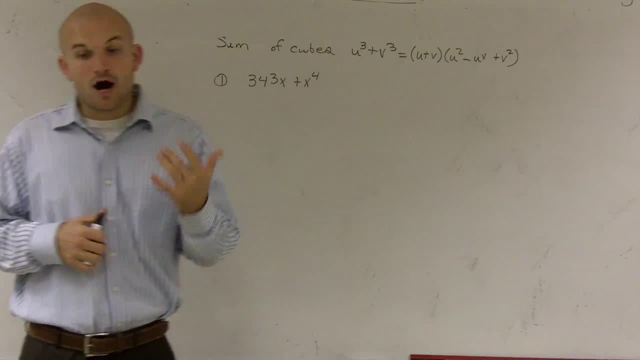 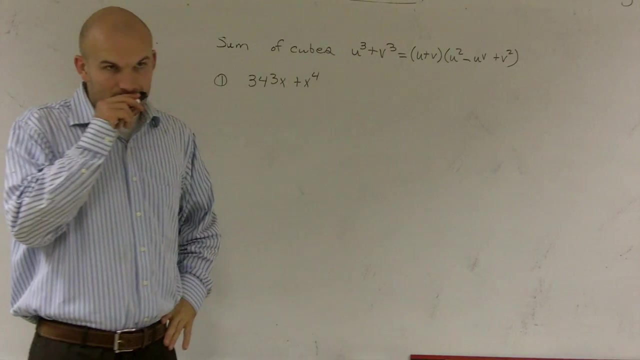 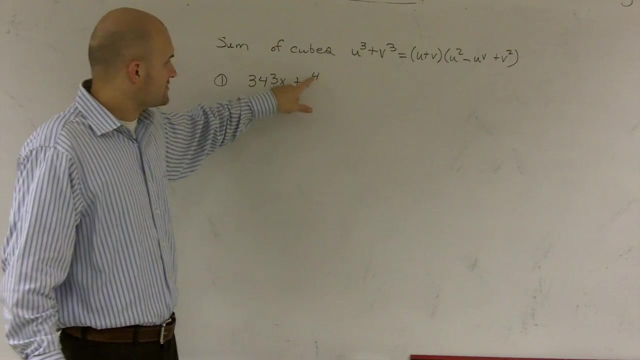 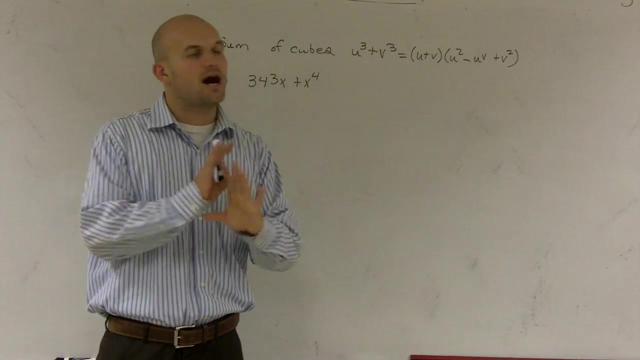 u squared minus u times v plus v squared. So automatically. what that's telling me is, if I want to use the sum of cubes, I need to have something that looks like this, And when doing that, I need to say: well, I don't have anything cubed, do I? First of all, I have an x to the fourth and I have 343.. Well, I do notice. I always, you always- want to look whenever you're factoring, always see what you can factor out right, Greatest common factor. So I can factor out an x. 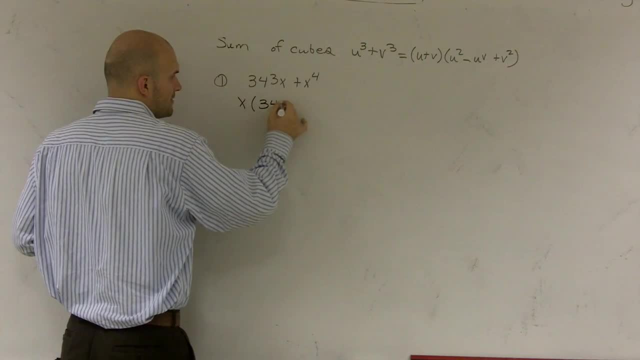 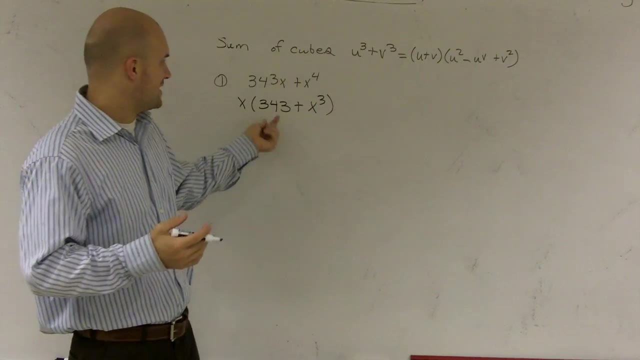 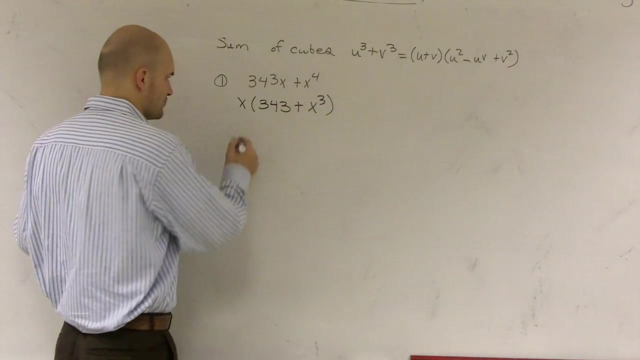 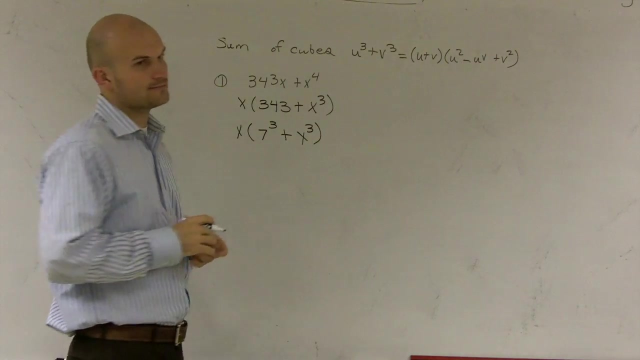 So I can factor out an x. So I can factor out an x. So I'll factor out the x here. So I'm left with 343 plus x cubed. Well, that's good. Now I got one x cubed. I need to see: can I write 343 as a number cubed? And just so happens I can. I can actually rewrite 343 as the number 7 cubed. All right, That's right, because I checked my calculator to make sure it works And since it does, it's perfect. Now what I can do is I can write 343 as the number 7 cubed. 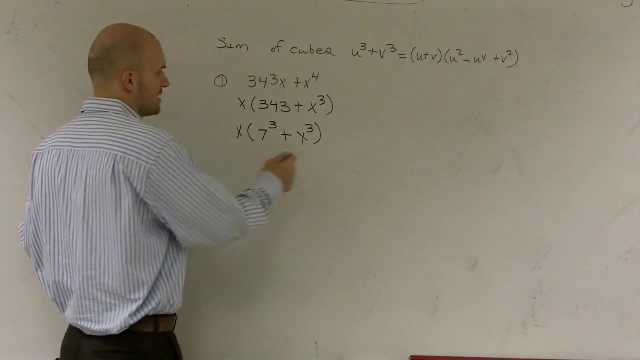 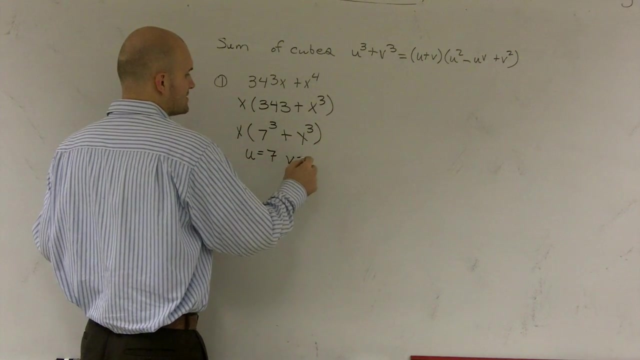 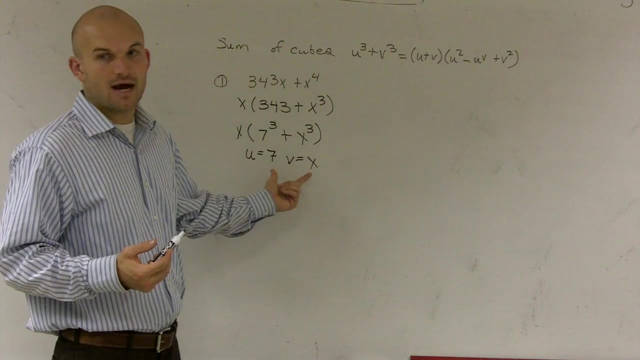 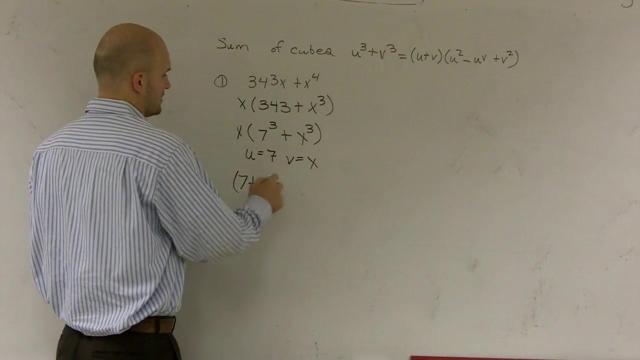 Now what I can do is I can use this formula. So now what I essentially have is u is equal to 7 and v is equal, or- I'm sorry- v is equal to x. So all I'm going to do is I'm going to take my values of this now and I'm going to plug them into the formula. So I say 7 plus x times 7 squared, which is 49.. 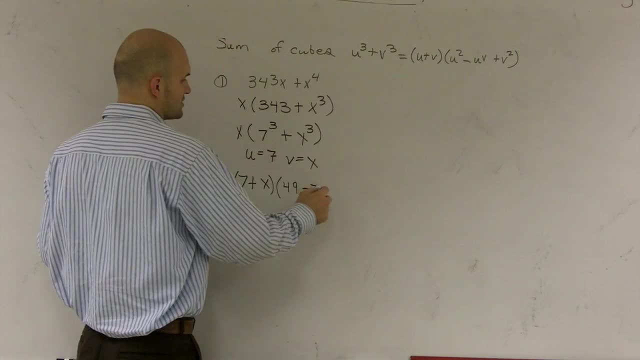 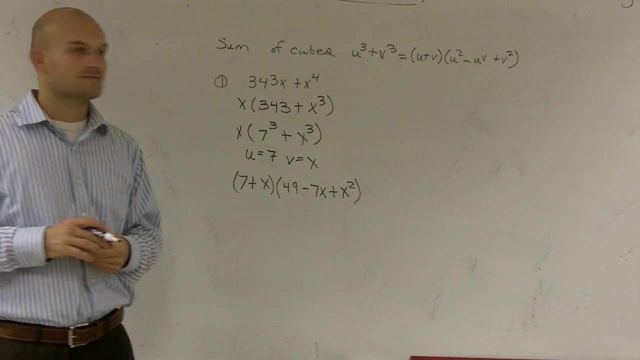 Minus 7 times x, which is 7x plus x squared, And that is now factored using the sum of cubes.